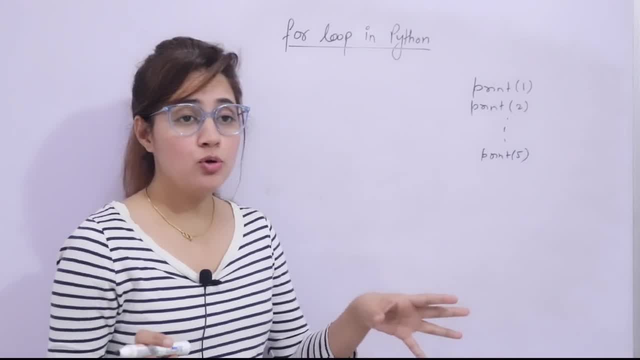 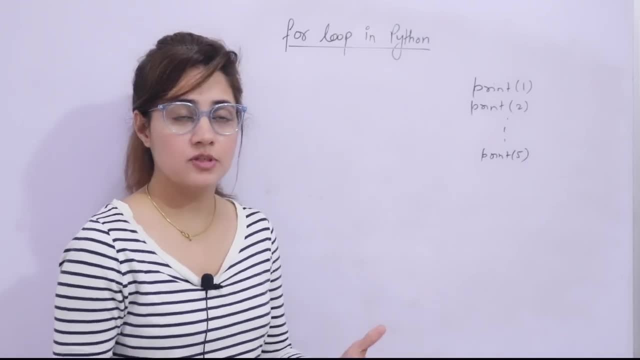 again and again. that is a loop, right? So in programming also we have to do These kind of task sometime. We have to repeat some statements or some instructions again and again. Some statements again and again, right? So you can put: so that is what a loop, So you can put those. 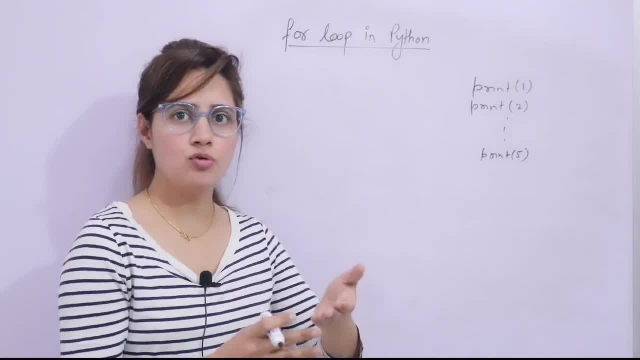 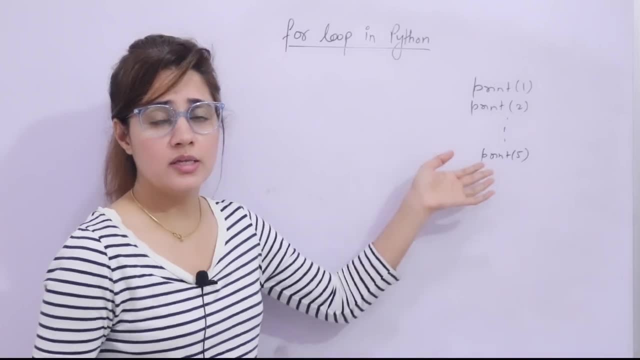 statements under a single line, like in a loop, And you don't have to write the same statements again and again. So this thing we can do with the help of loop. How That also I'll tell you. In that case you need to write down the sprint: only single time, like one time, not five time. 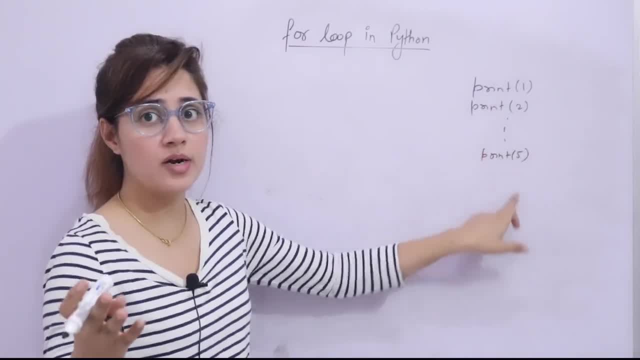 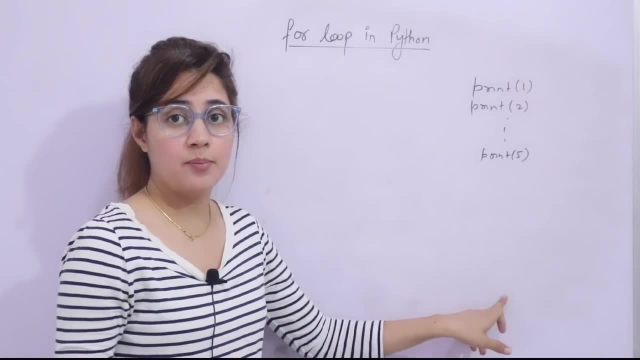 Because, yeah, that is fine, You can write down print 5 times, but if I ask you to print 100 times, 1 to 100,, if I ask you to print 1 to 200,, 1 to 1000, so it is not possible to write down 1000 time print statement and that is. 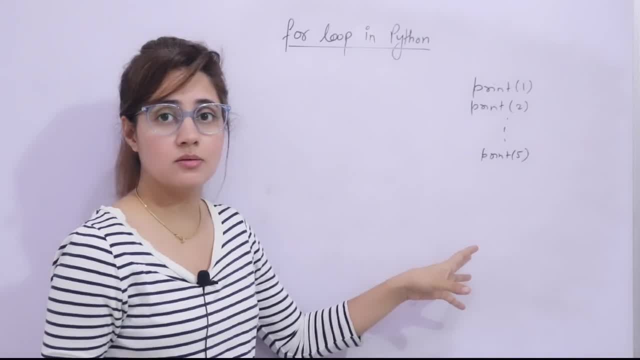 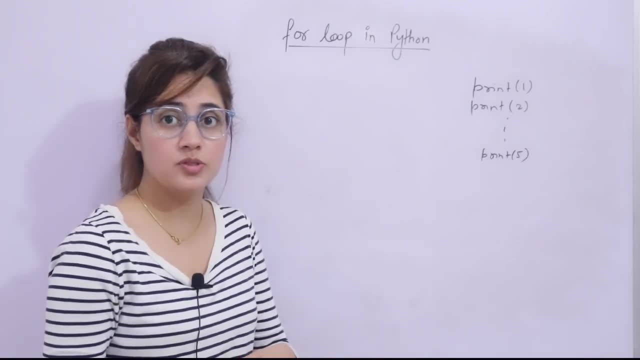 obviously a, you know, waste of space, right, And waste of your time, right? So better to use loops in Python for this thing. we have loops in Python, Basically two types of loop: for loop and while loop. Third is also that is nested loop. nested means what? Within? 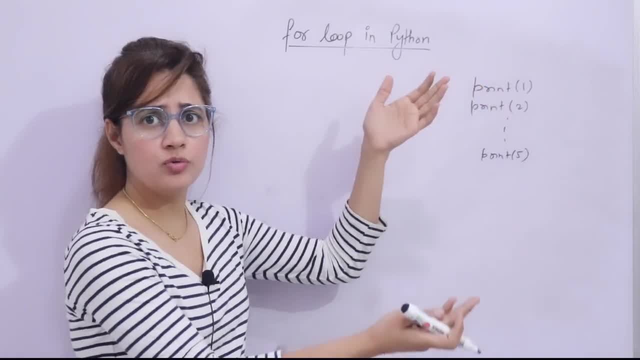 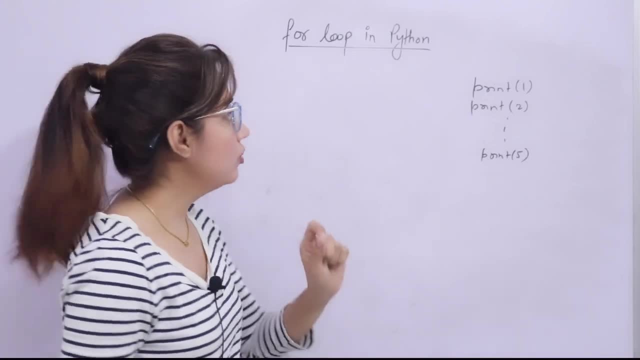 loop within a loop, like you are, you have written a for loop within that loop, you have written again a for loop, or maybe a while loop, right? That is what? a nested loop, but mainly two types of loop: for and while. So in this video we will be talking about for. 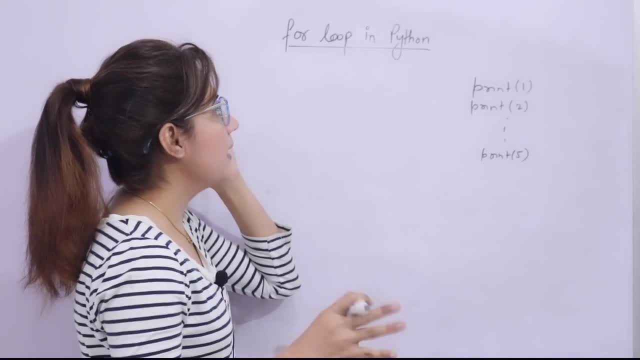 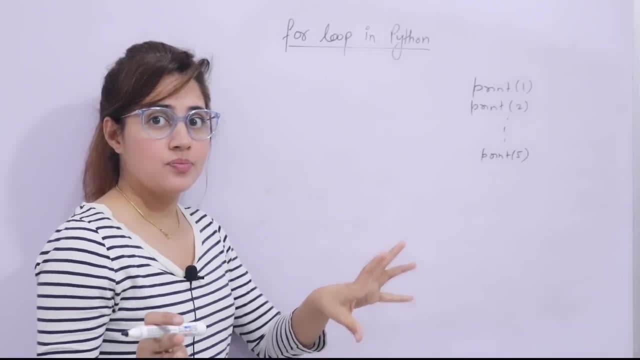 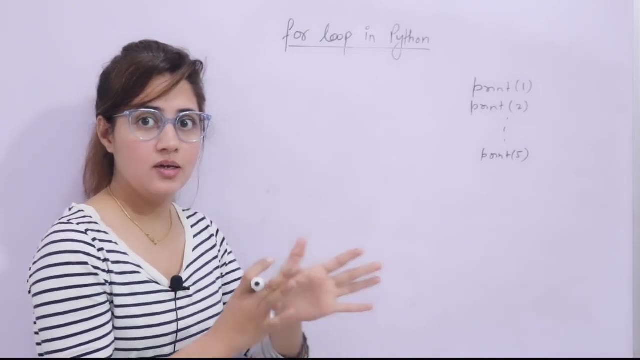 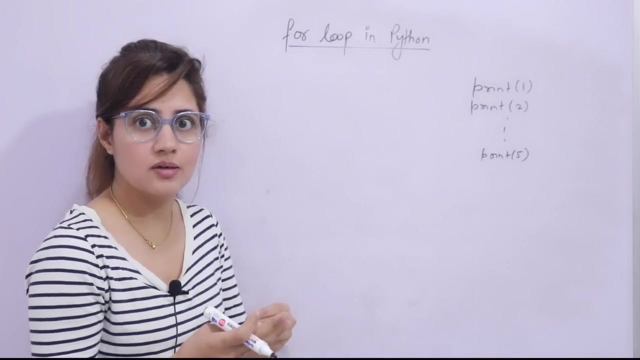 loop. So here for loop is what In Python basically, maybe if you have read for loop in other languages- C, C++, Java- then it is not the same like we have discussed in other languages. right In Python this for loop is more like an iterator. Now what is iterator? Iterator is you can 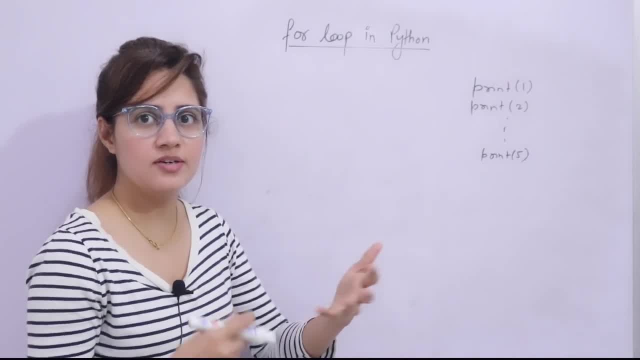 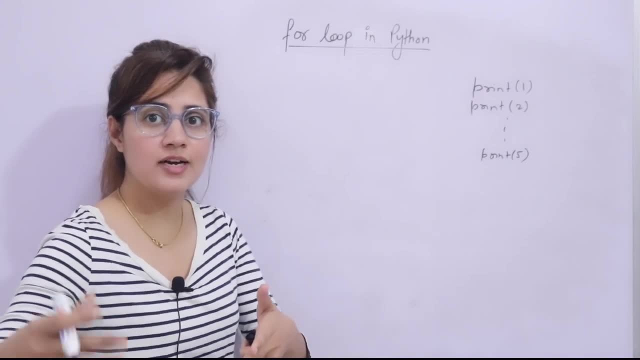 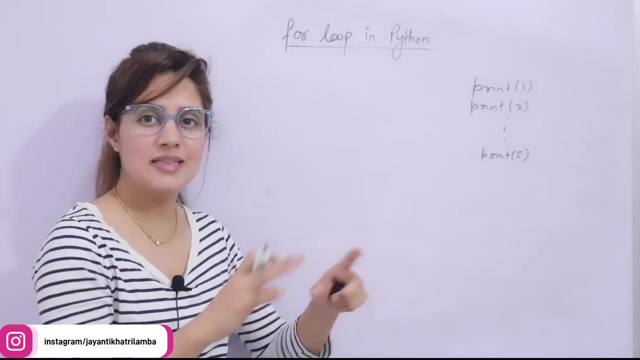 say, which is used to do some iteration. Iteration is what? Traversing a sequence 1 by 1, traversing a sequence 1 by 1, that is called iteration Sequence. here is what now. Now, sequence in Python is what Collection of items, sequence, data times, or what List, tupperware list? 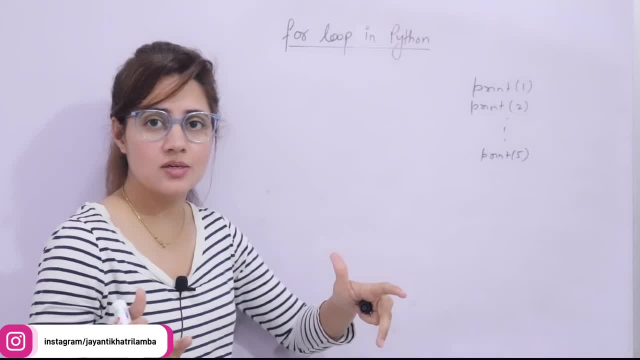 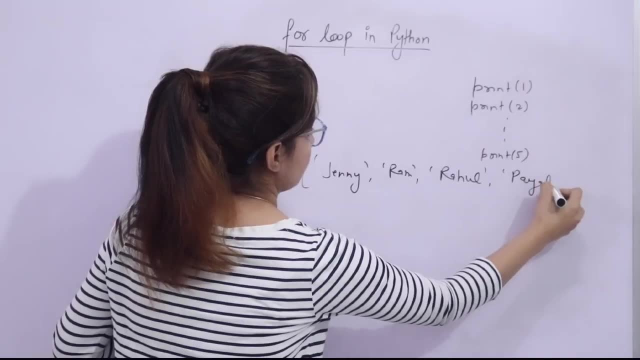 list, list. So this is what we call set dictionary. that we haven't discussed, we will be discussing later. String is also a sequence, So like this: if we have a list, something like this, if we have like four names, so this is a list, or you can say this is a sequence collection. 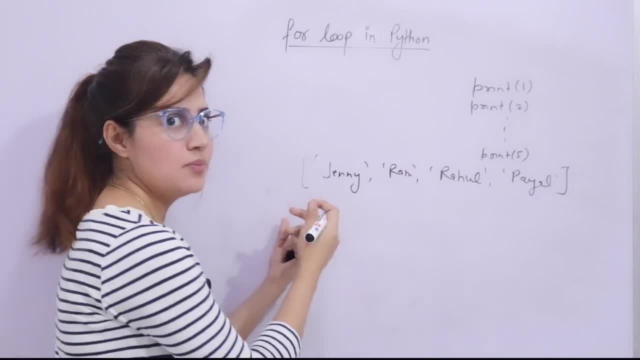 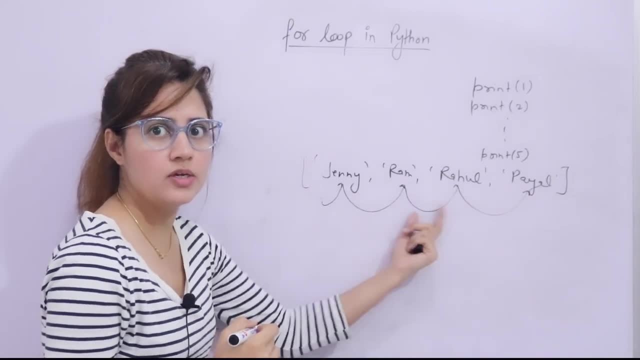 of items, right, So traversing of this sequence. traversing means go to first item, then second item, then third item, then fourth item, like this. So this is what traversing, this is what Iteration, and using iterator we do this iteration. So that is basically in Python. 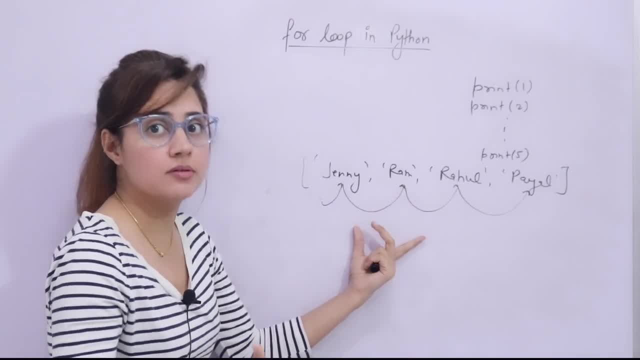 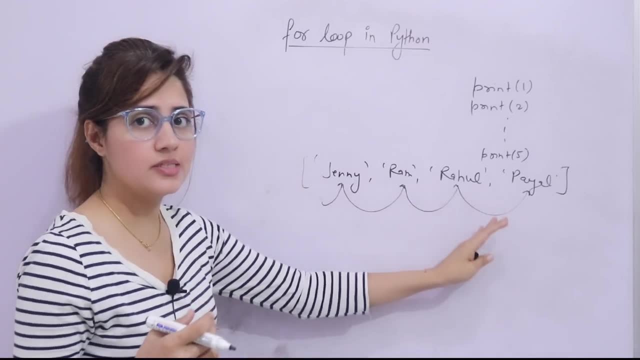 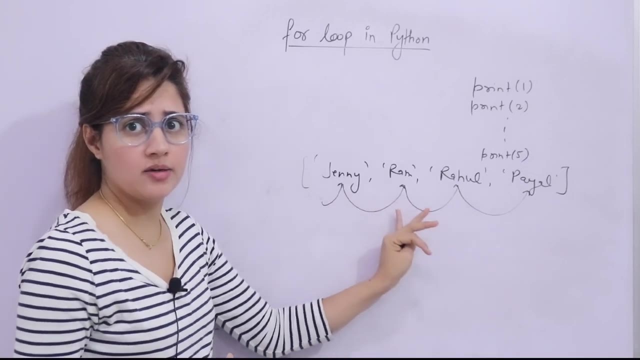 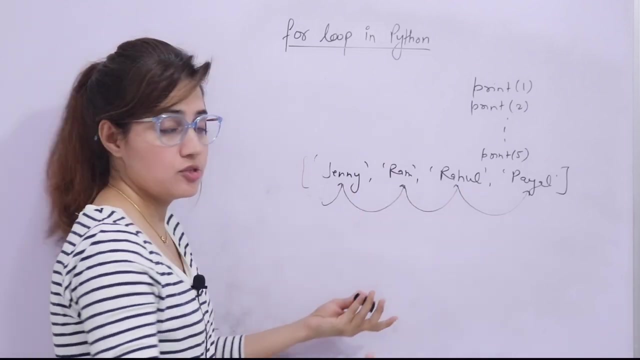 for loop. For loop is more like an iterator right. So we can say a for loop in Python is used. used to iterate over a sequence in Python right And do some specific action for each item, or you can do some specific action on each item in that sequence right. 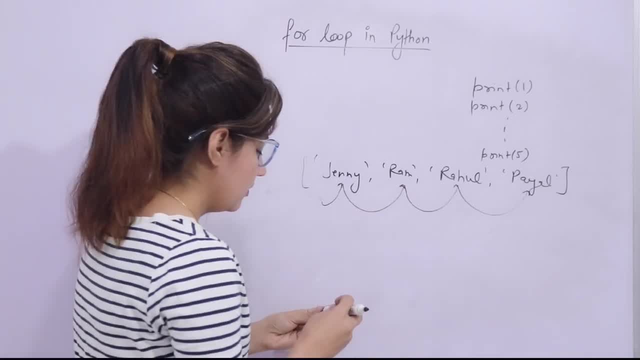 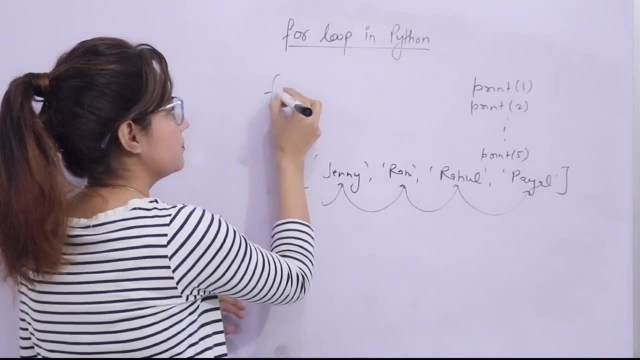 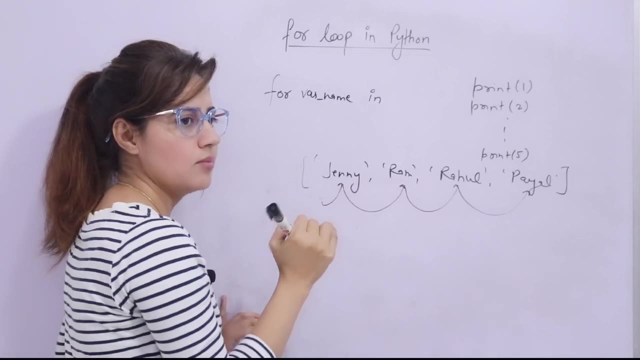 Sequence may be a list or a set or a tupperware or a string or a dictionary. Let's take one example How you will. let's see syntax of for loop. You simply write this: for we will be writing a variable name here, any variable name in membership operator, not in and in. we have 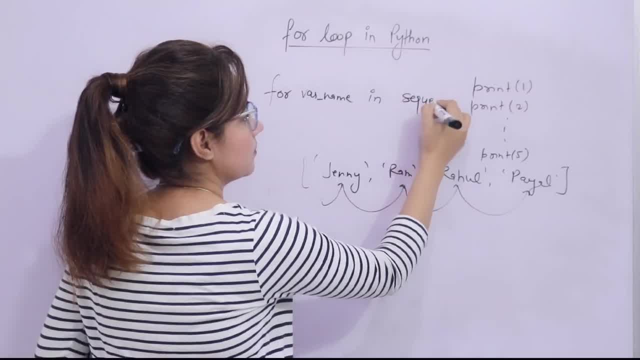 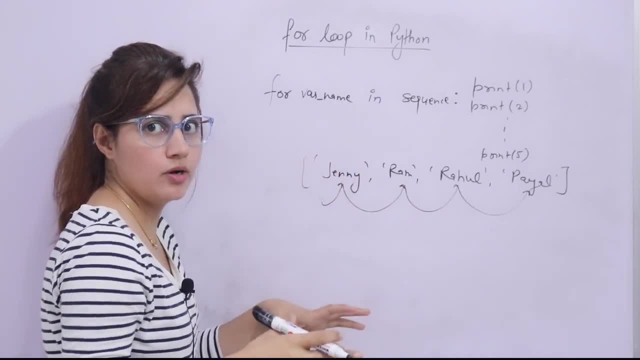 discussed in here. you will write that sequence name, sequence then column. sequence may be a list of this name or a tupple name or whatever. you have taken that sequence name And here you can write down those statements. Okay, 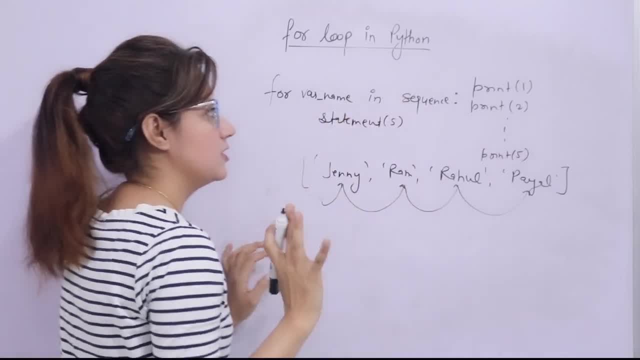 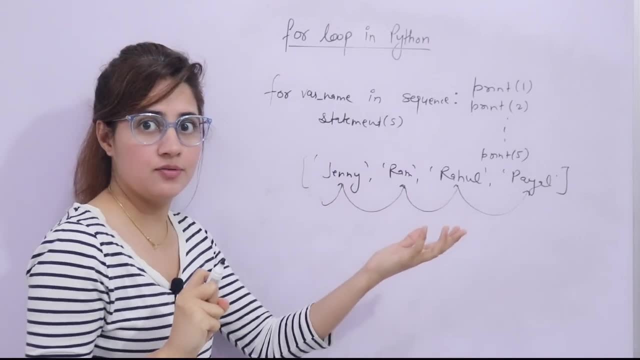 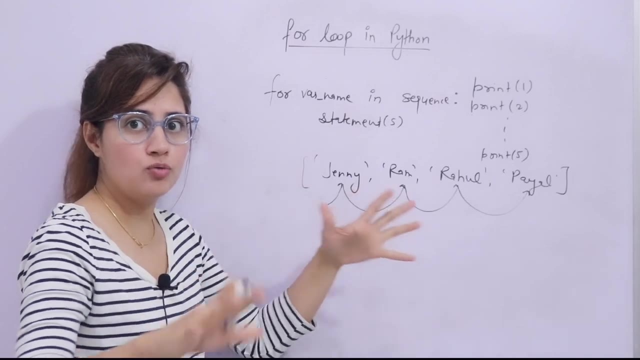 One statement or multiple statements can be there. This is simple syntax of writing a for loop. There is no specific condition like in other languages we have. we have to initialize for loop, then we we giving some condition, then increment, decrement and all So nothing. 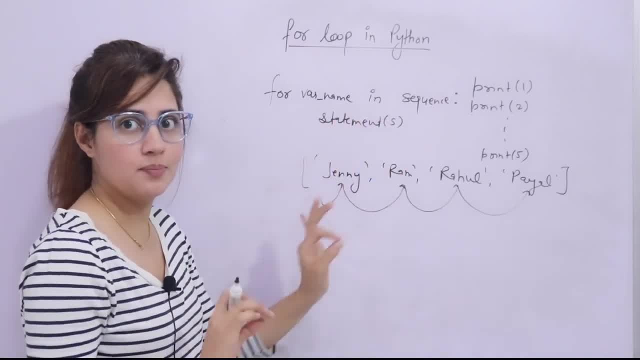 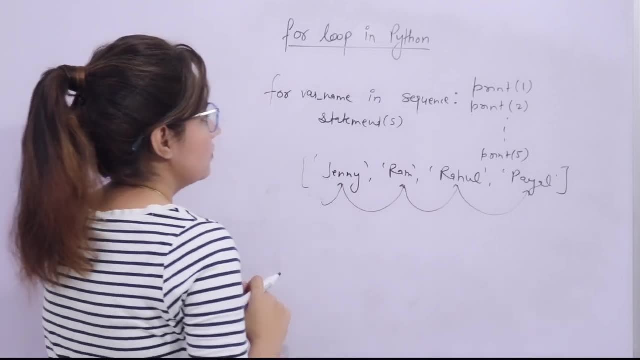 you have to specify. that's it you have to do in Python, right? You don't have to initialize any way like variable name or anything. Fine, Now in this case, suppose you have to write list number, so this méthode makes the больше comfortable. Suppose I have this list List. 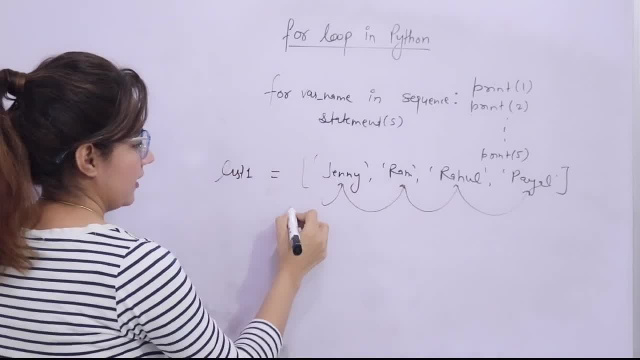 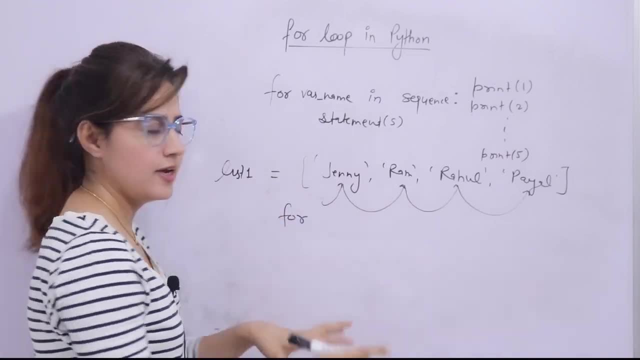 number. So it says: list one, List one is this. So what you will write, like four: you variable name, any variable name you can take, like I, B, C, D, X, Y, any of them. So 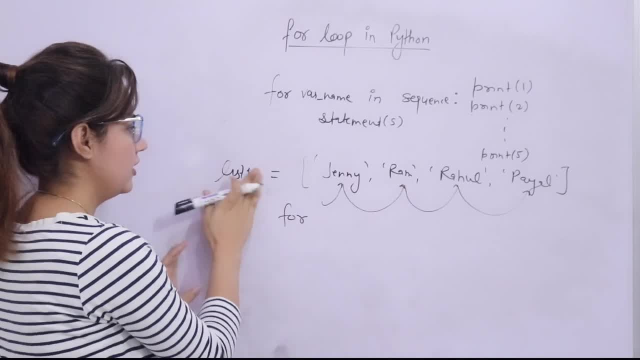 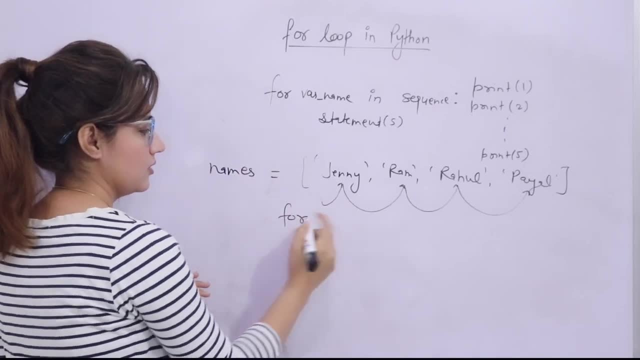 if these are names, right. or you can say here also you can take a that meaningful name names list name is names, So I am taking a meaningful variable name also Four, let's say four multiplic bodily. Did you see? Just order to get then whatاي believing that? 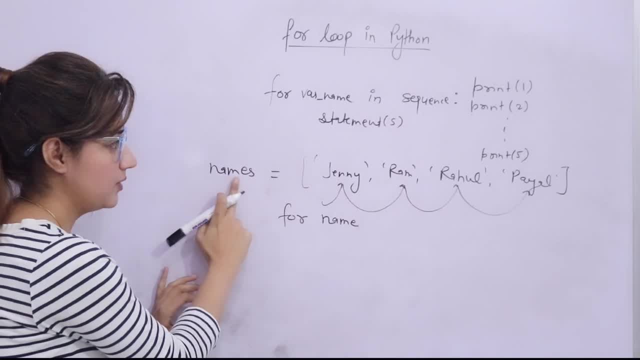 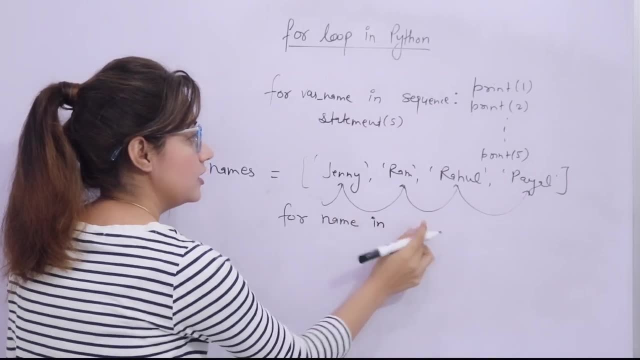 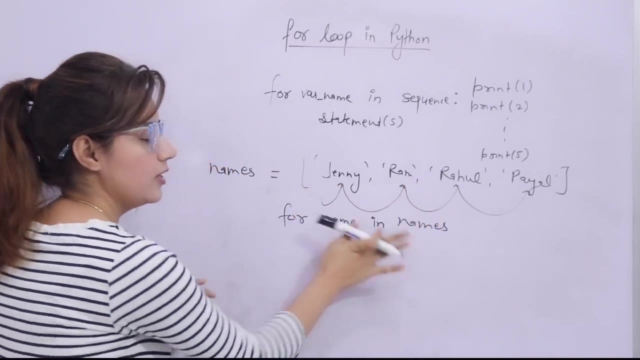 name, not the same variable name that you have taken, the sequence name. that should be different. Here we have names. here we have name For name in sequence name is what Names For each name in names. what you need to do Here, you can do whatever you want to. 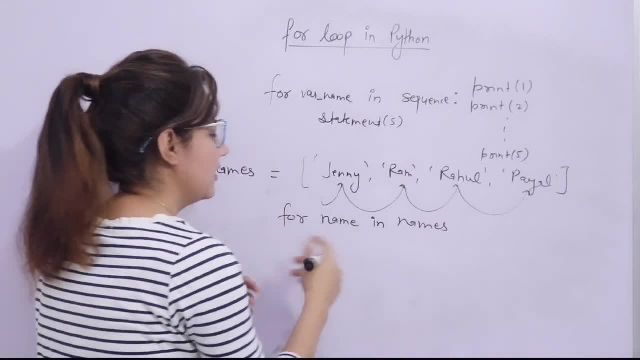 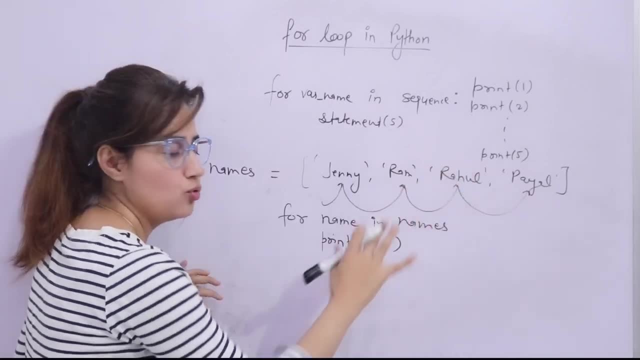 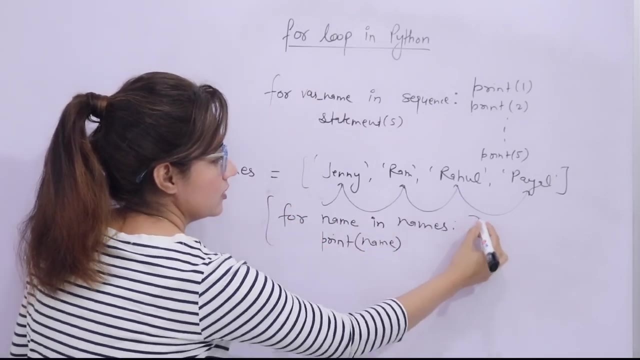 do. Simply, the very basic and simple thing is: I just want to print, So print, and I just want to print each name After traversing. I want to print each name, So print this variable name you have to write down here: Print name. that's it. Okay, I forgot this. 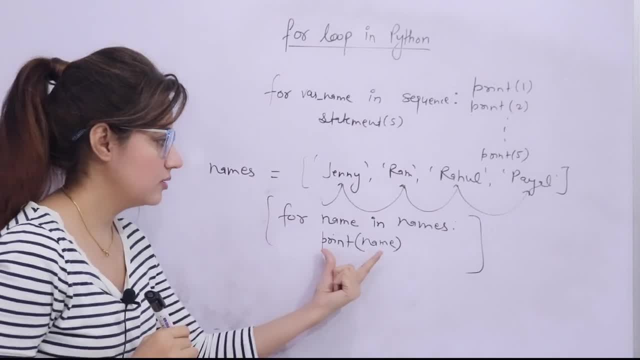 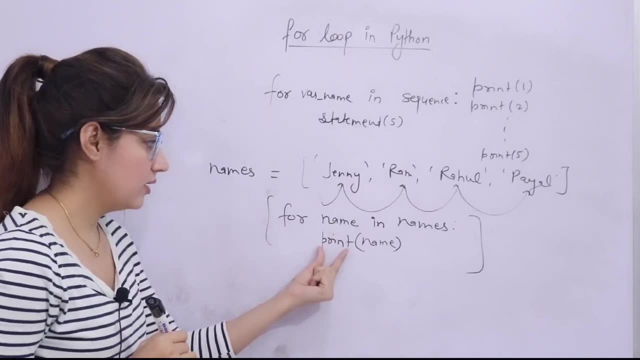 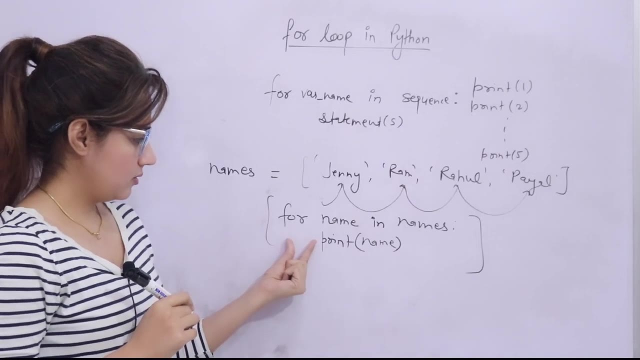 semicolon And please this statement would be indented. This indentation is very important, Otherwise it will give error. You will, if you write them, print here here without any indentation. it will give error Right. So better take some indentation here. Now what? 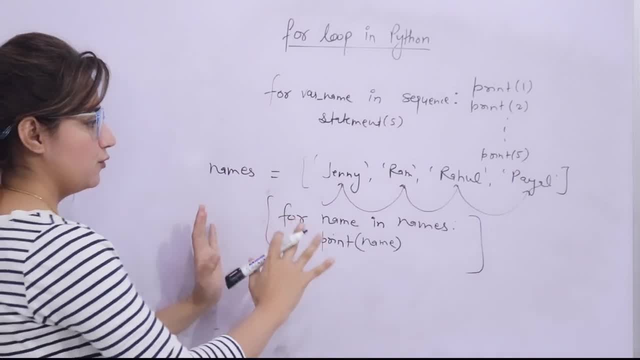 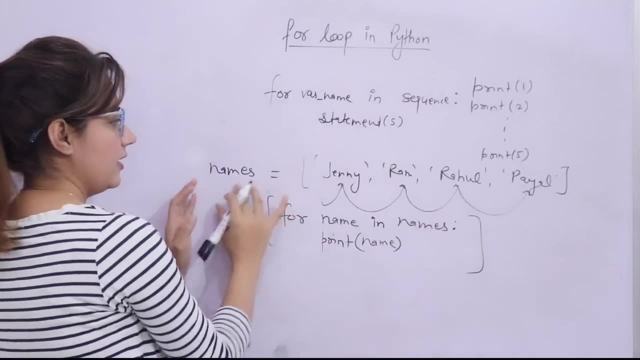 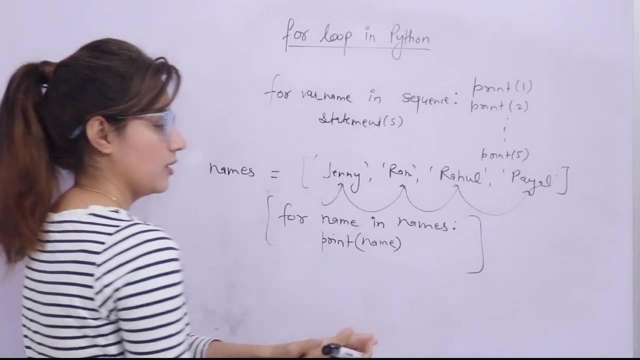 it will give. What is the working? First names is what This? So it would be here, This complete list would be here, Or rather than this directly here, Rather than names directly, you can put this list here. That is also fine. So now, first of all this: what is the internal? 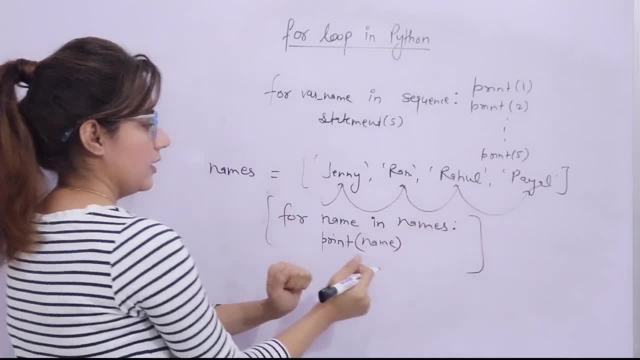 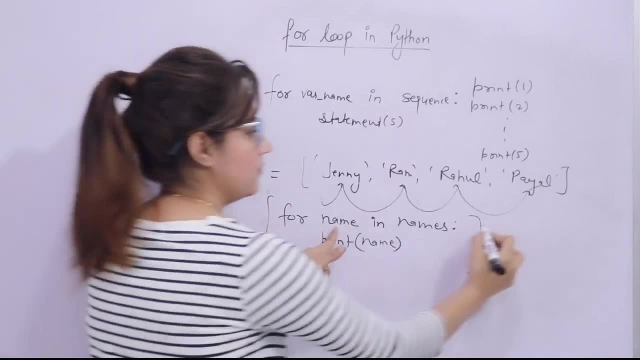 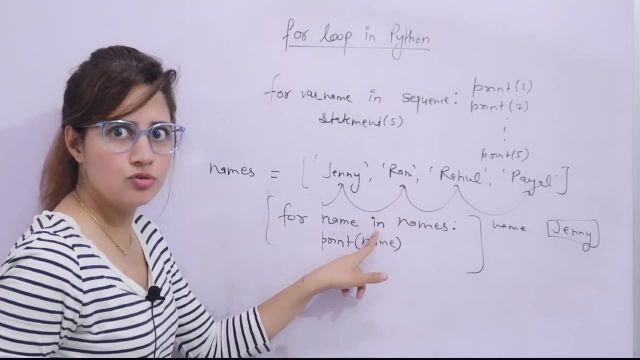 working. This names would be replaced with this list. Now for name in names. first name, Jenny, would be assigned to this name. This is a variable name or a placeholder, So in name first we have Jenny, For Jenny in names, so condition is true. In operator membership. 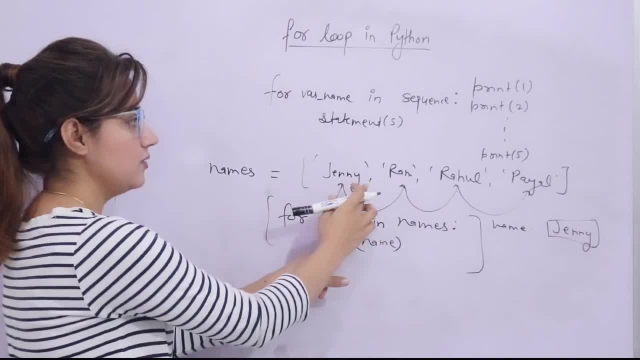 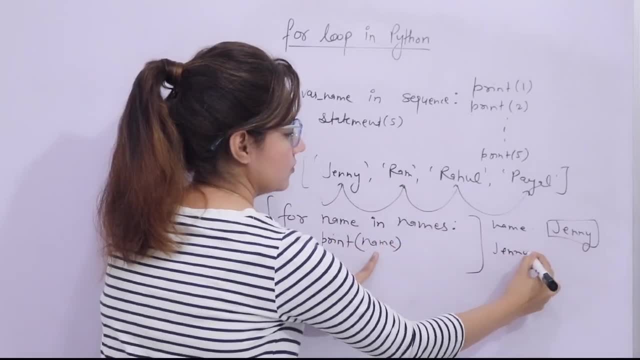 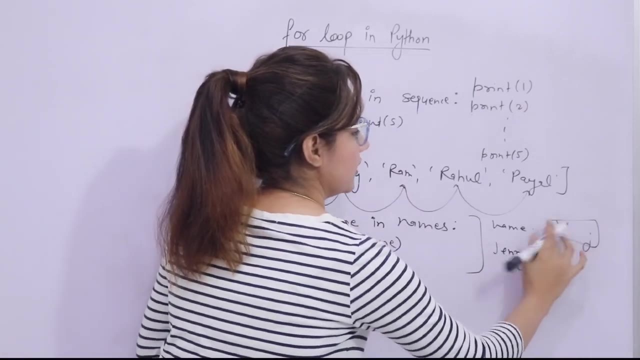 operator that will give, because Jenny is present in this list names, So it will give true. So enter into for loop and print name. So in name we have Jenny, So it will print Jenny now Again. now next is Ram, So next time Ram would be assigned to this name. 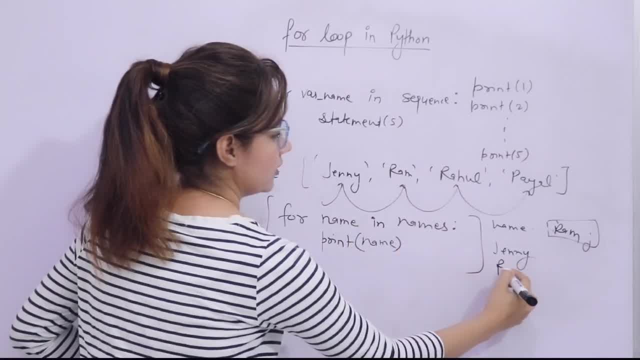 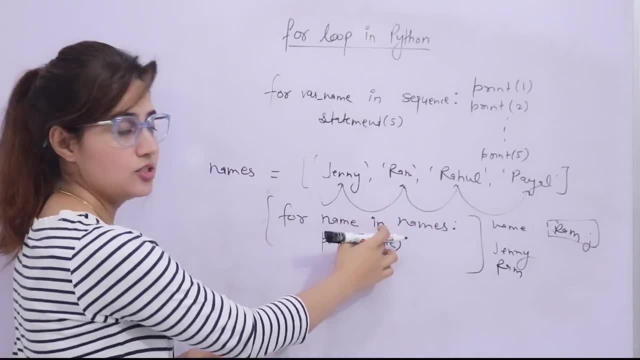 Ram in names. yes, true Print name. So next line, Ram, will be printed like this. Next time, Rahul would be assigned to this name. Next time, Payal would be assigned to this name. All the conditions are true And we will print Till the end of the list. it will. 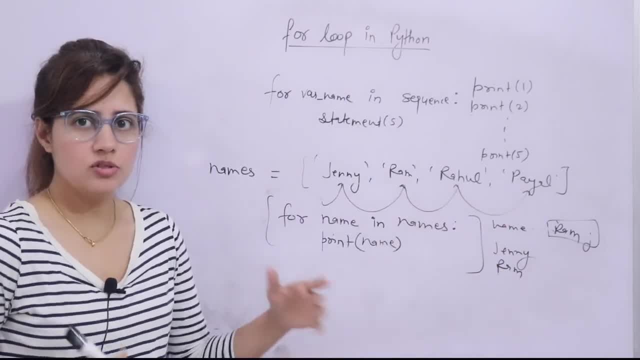 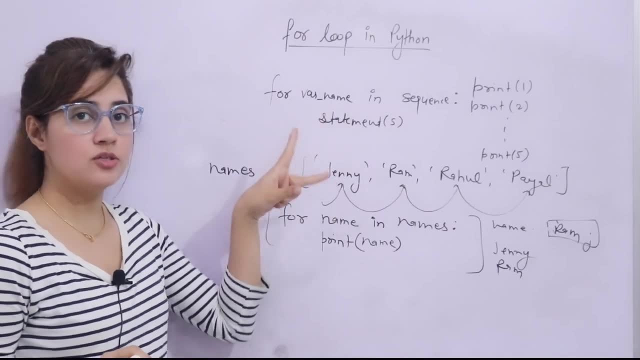 print all the names: Jenny, Ram, Rahul and Payal, something like this. So this is simple working of for loop Right. It will do these actions. whatever you will write here, It will execute these statements for each item in the sequence. Sequence may be placed or: 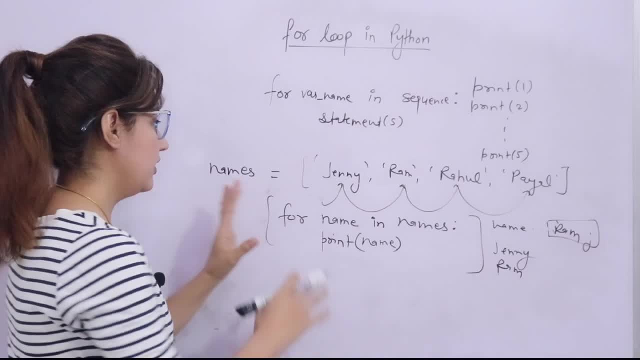 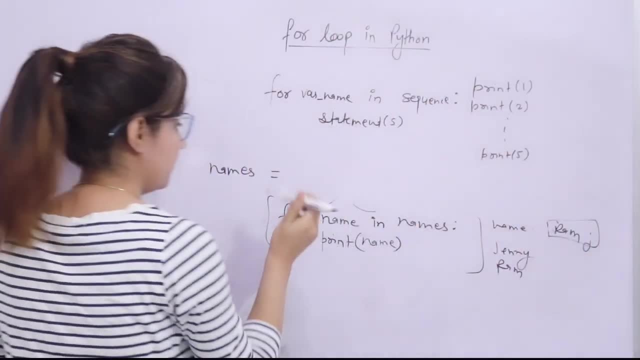 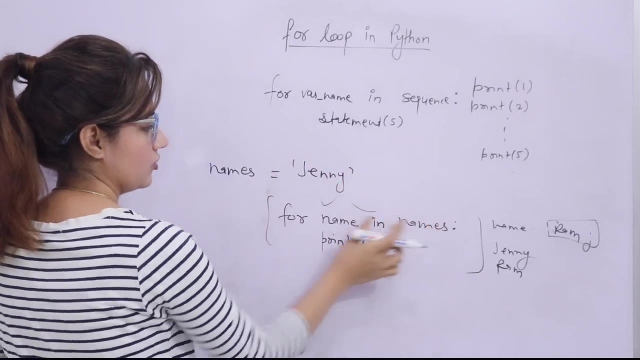 tuple or set Right, If, rather than this, if you simply take string, then also it will work. If I simply take this string, Jenny, this is also a sequence. So in names now we have Jenny string In name, now what we have First time we will have J, So J in names. yes, So it. 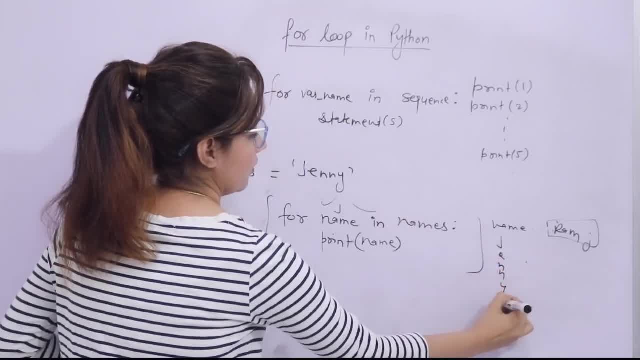 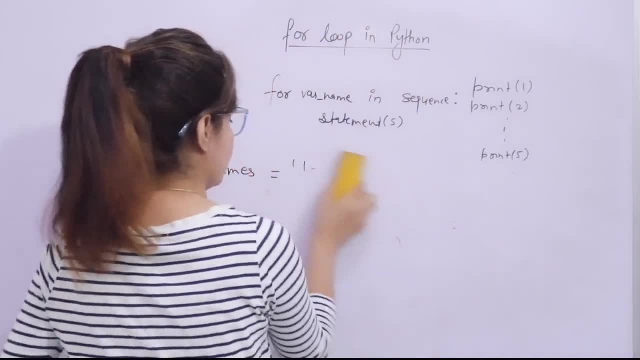 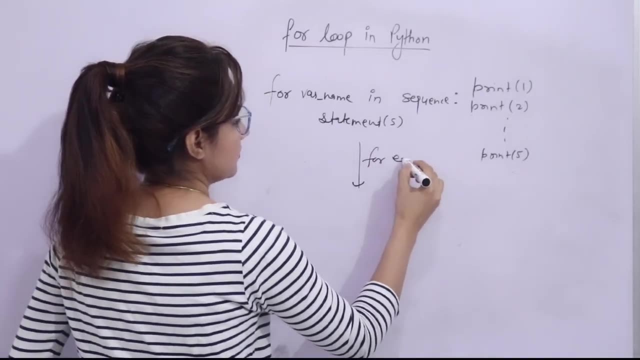 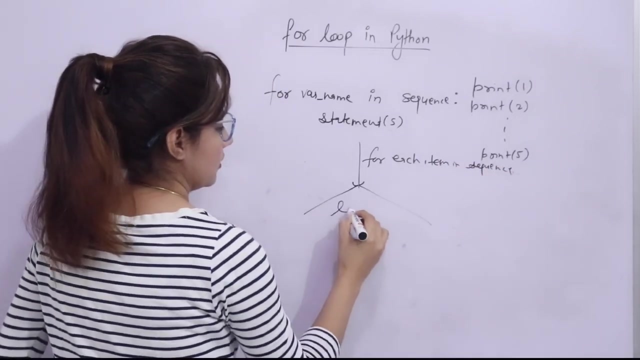 will print first J, then E, then N, N, Y, something like this: Right, So if we draw flowchart, or simply if we try to draw flowchart for the loop, then that would be like for each item in sequence what it will do: Last item reached. If this is true, then exit from previous. 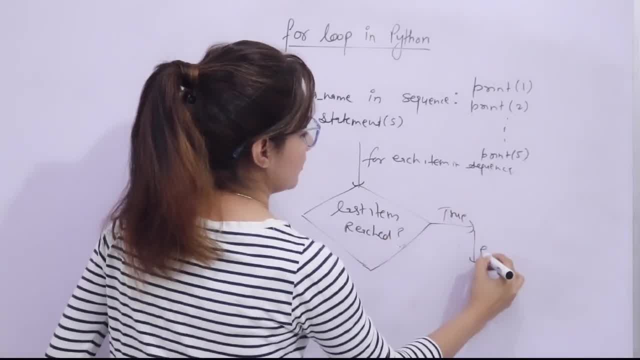 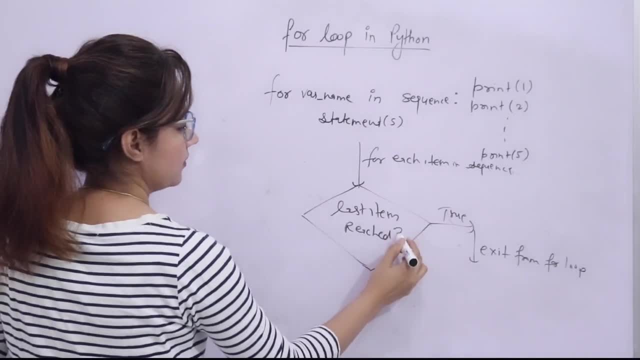 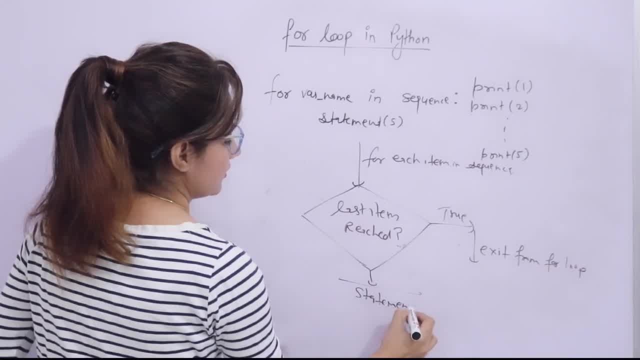 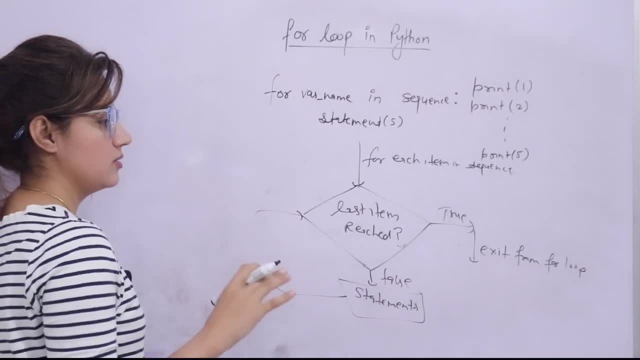 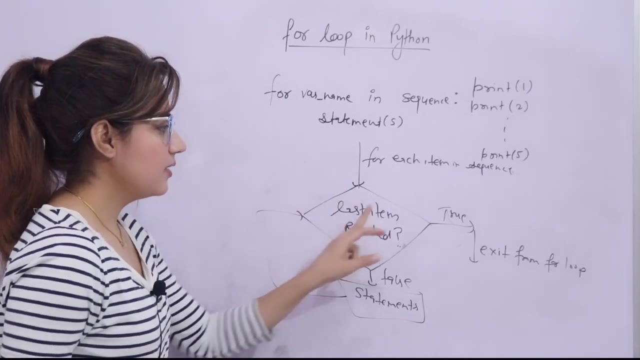 then what it will do. Whatever the statement is there, that would be executed if this is false and then again will be here. So this is kind of flow chart. you can draw for this for loop in Python, right. Once last item reached, exit from for loop. I have told you. 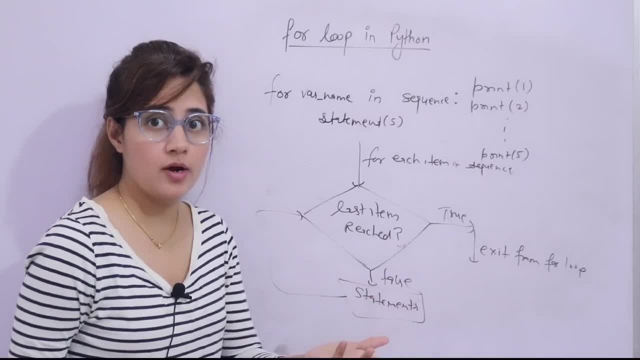 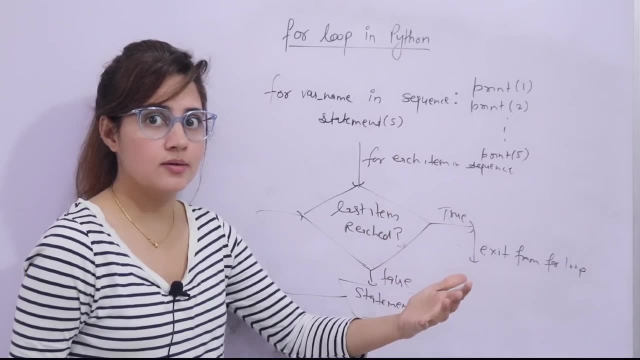 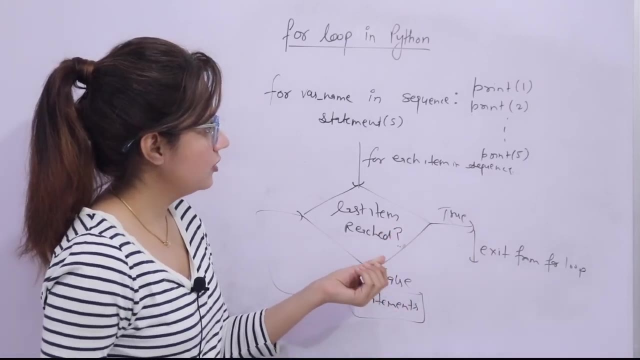 it is more like an iterator method that we find in other object oriented programming languages, not more like for loop, right In other languages the for loop is there. So not same that for loop, but it is more like an iterator, means we execute these set of. 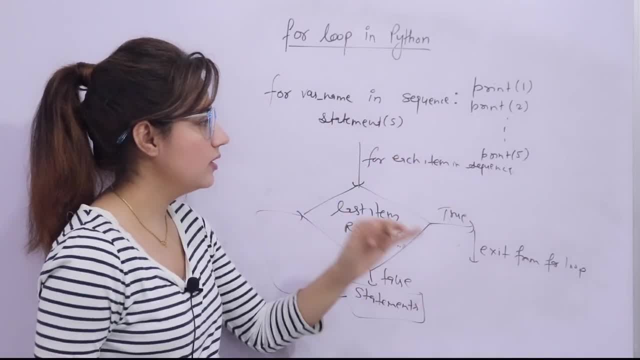 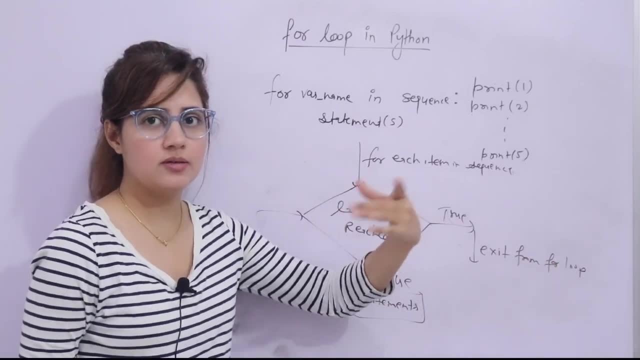 statement once for each item in the sequence. right Yeah, but also how you will print like 1, 200 and 1, 2, 200. that also we can do. for that. we have another method In function here, that is range function. So you can use range function for loop and you 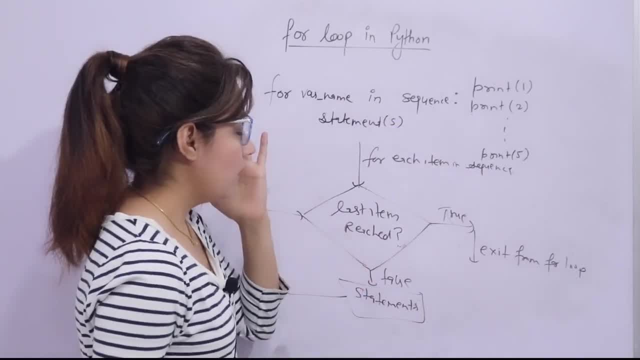 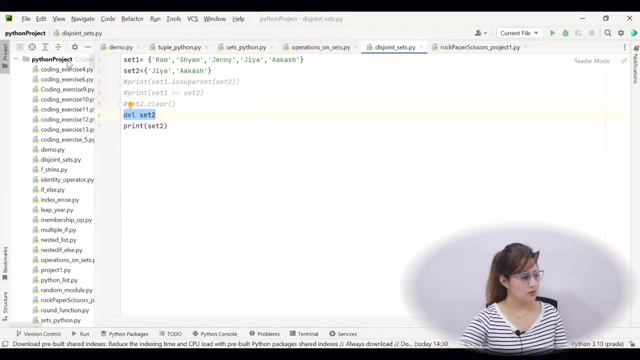 can print the numbers also. right Now let me just show you this thing with the help of practically, we will see like program. with help of program, I will show you. Okay, so let us create a new file here. I will be naming it for underscore loop dot. 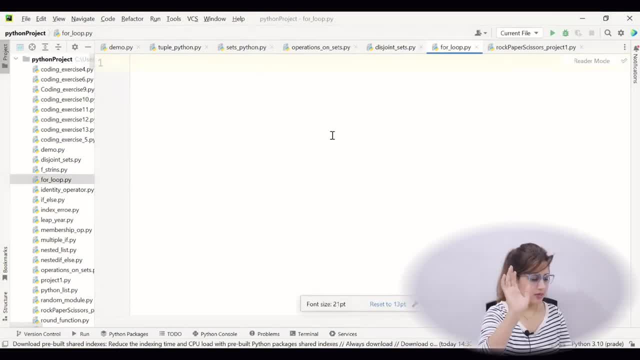 py. right, Okay, simply, first we will take any sequence. Let us take any sequence. Let us take any sequence. Let us take a list. Why always list? Let us take a string only. So I will be taking like name, equal to, and here I am taking Jenny. that is it Now, for let us take a variable name. 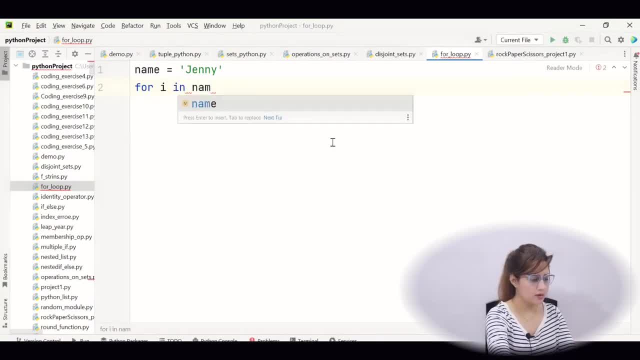 Let us take I, any item you can take for I in this name, then colon, and you simply want to print. that is the simplest action we can do: print, But you have to put here variable name. I right, Let us just run this and I will show. 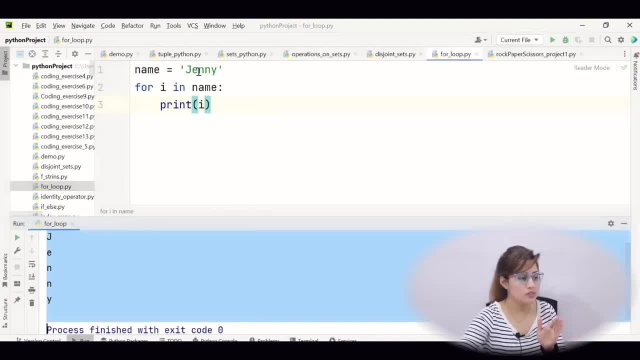 you C, j, e, n, n, y. you have traversed this sequence using for loop. that is what iterator do, right, Iteration traversing a sequence, and this statement can be executed once for every item in this, this sequence. So this time I will be taking list. So now, this time, 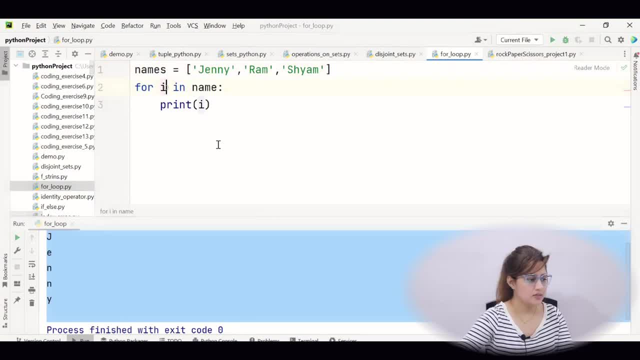 we have names. Yes, Yes, this list and same. you can do with this If you. you can. just variable name is: i is fine, let us run this and this time see Jenny, Ram and Shah, right, But within this you can also. 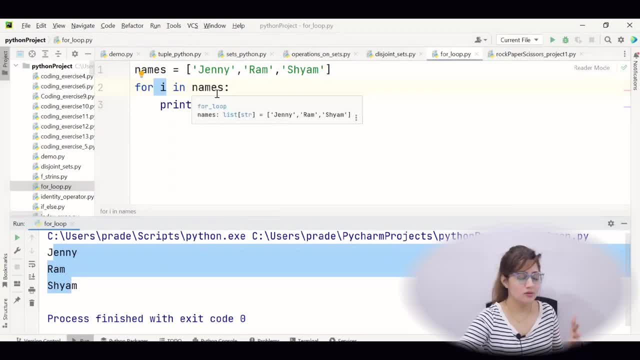 this is what the simplest thing we can do, but we will use it during more complex actions and within this, not exactly one statement, you can write multiple statements also. right, and see the indentation part. that is very important. if you do not put here indentation, that is by default actually, because, see, whenever after this i enter, then cursor is here by. 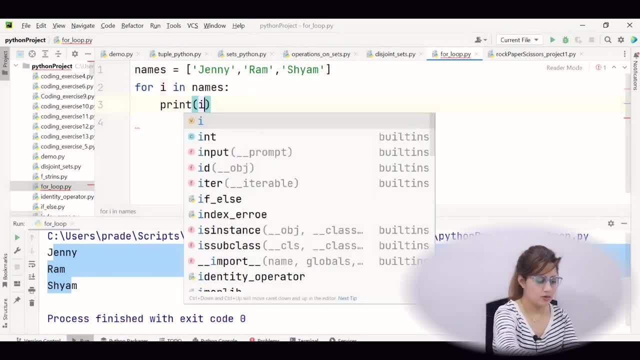 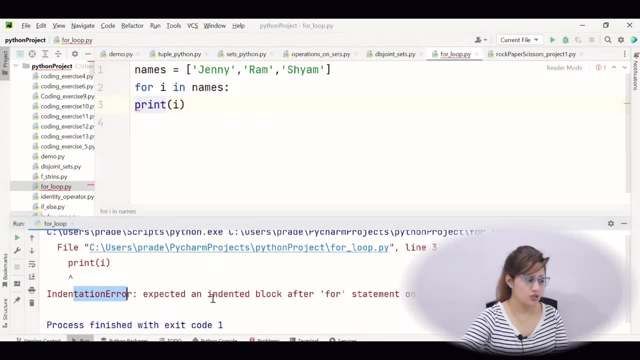 default indented. so simply like print, right. but if you do not, if you remove this indentation, that would be an error, see indentation error. expected an indented block after four statement in line. So we have to be very careful about this indentation part because this will specify a block. these 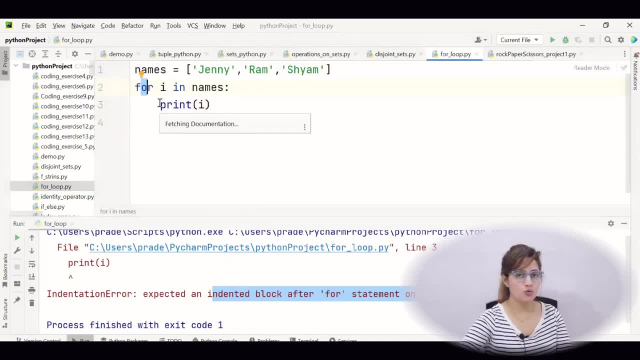 whatever statements are indented that are under this for loop, right In COC++ or another, the languages for representing the block. we use curly braces right, but here we do not have such kind of thing. Simply indented means this is under the for loop and this is a block. 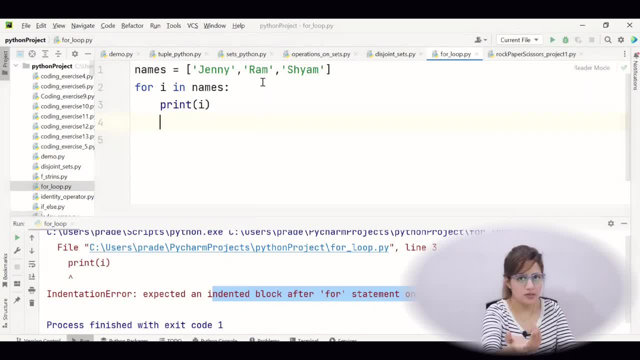 So, rather than this, we can also here print some other thing. we can also print some other thing. So again, we can also do like: if I print some condition, if this i equal to equal to jenny. if this is the case, okay, so jenny is a string, so we must put the same here. this is the case.